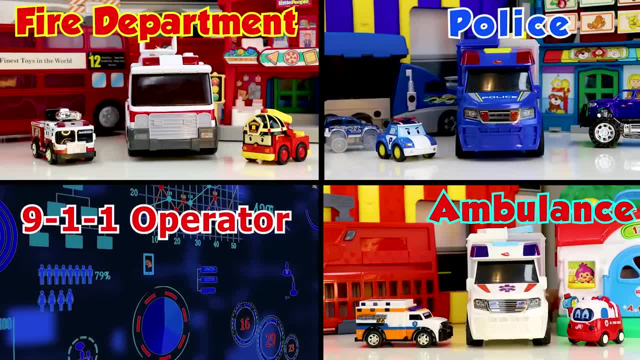 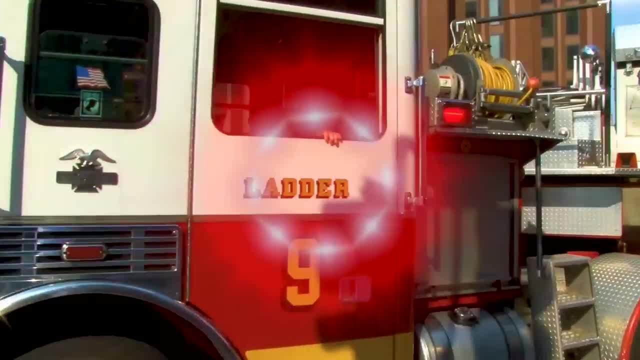 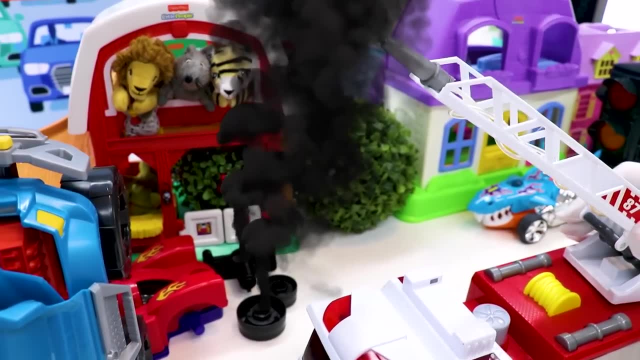 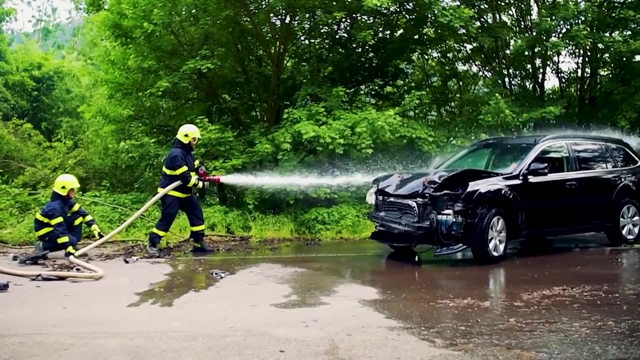 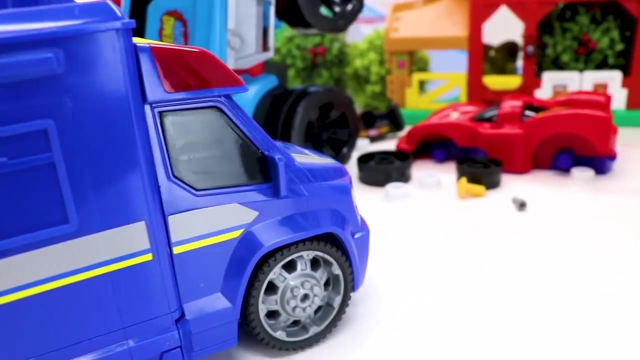 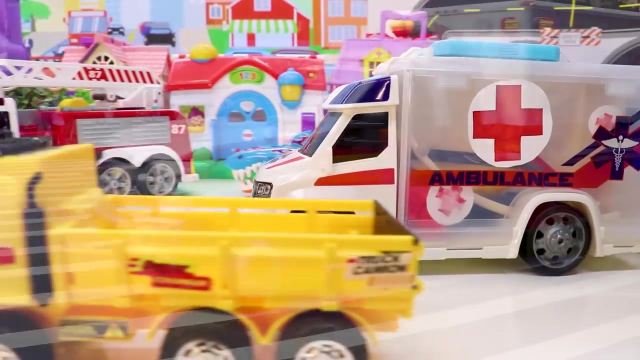 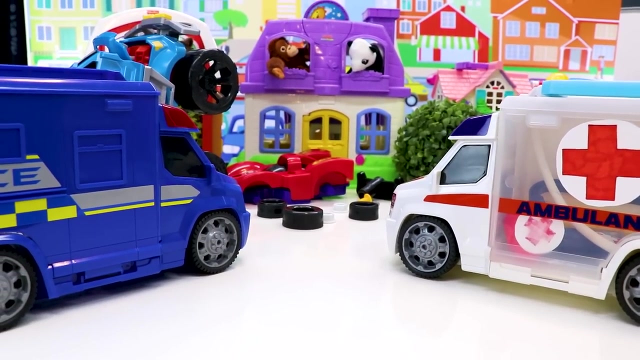 All emergency vehicles are to be dispatched. We're on our way. Help is here, Don't worry. Okay, I'm coming Police car here. Who needs help? I'm okay, We gotta check on a race car Ambulance here. Is anybody hurt? 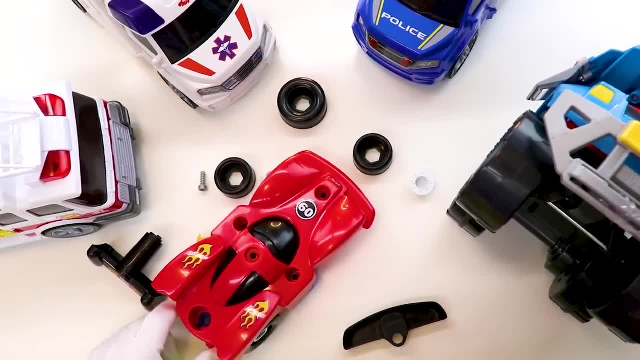 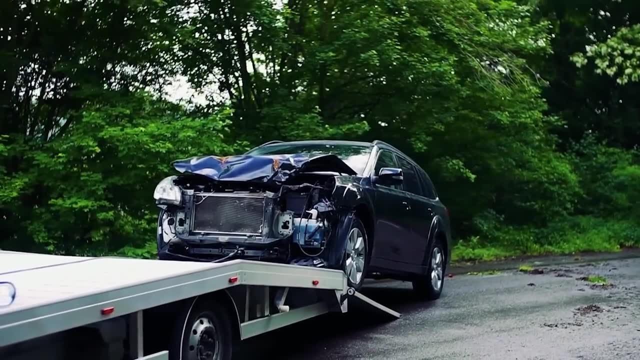 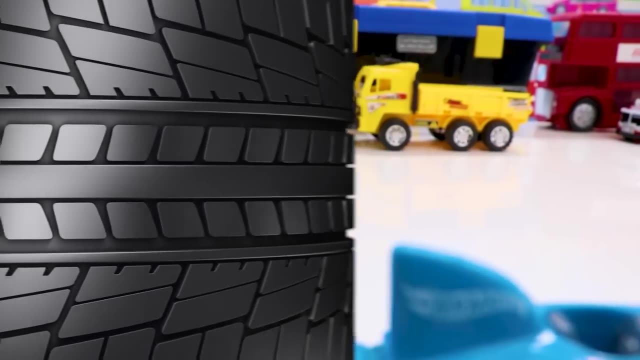 I'm all right, but I do need a mechanic. I'll call you both tow trucks and then I'll come to investigate. Requesting two tow trucks Immediately two tow trucks. Tow truck, tow truck. who called a tow truck? 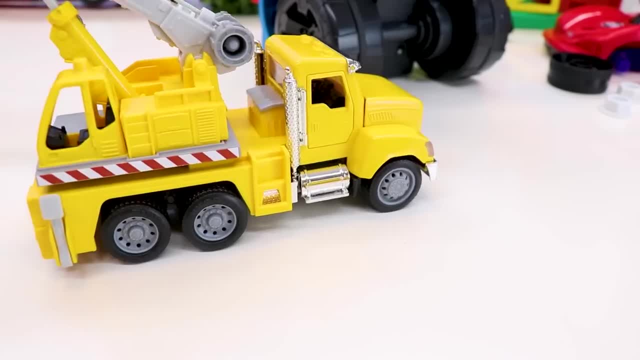 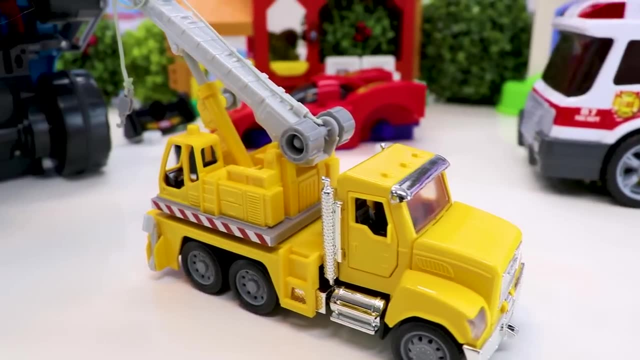 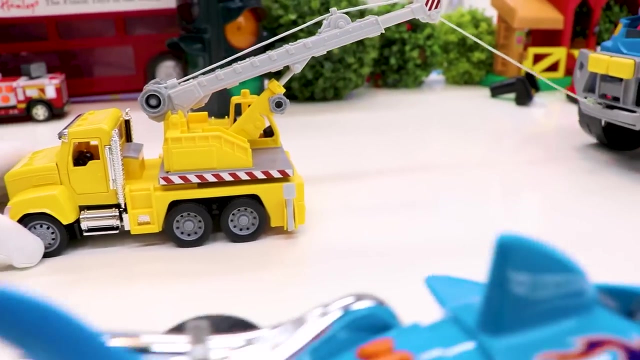 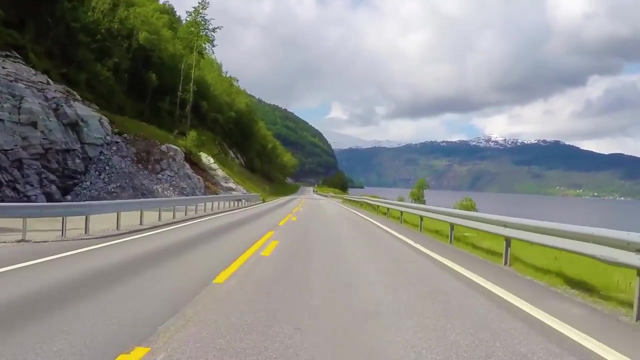 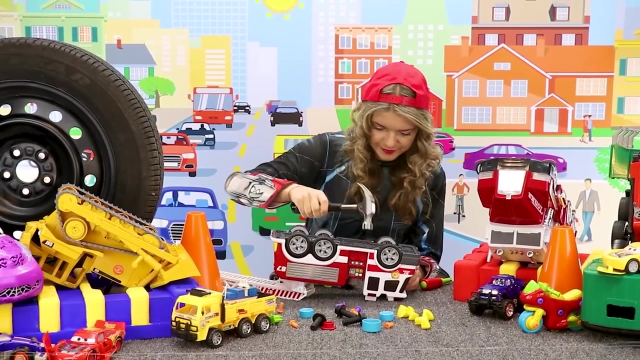 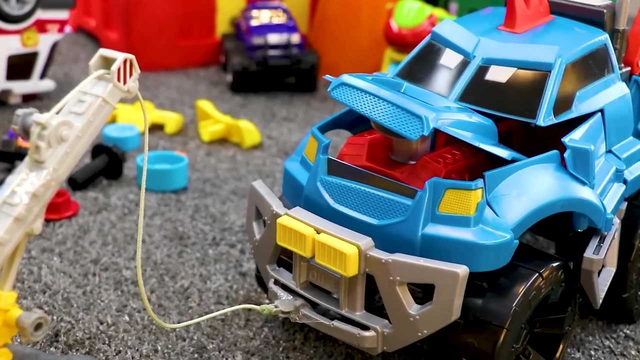 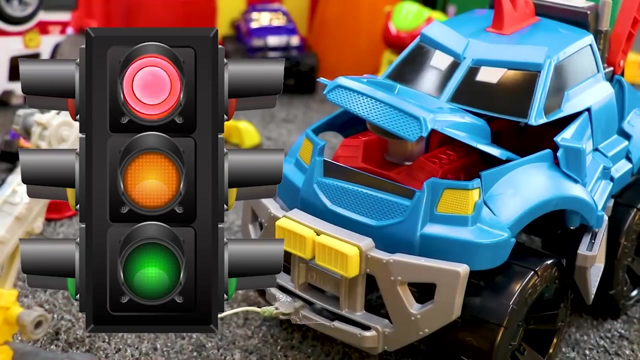 Great. Could you please help me down? Oh yeah, Off we go, Bibi, I have a visitor for you. All right, bring them in. Oh, careful, careful. Oh no, Demo Duke, what happened? I was going way too fast and I didn't see the red light. 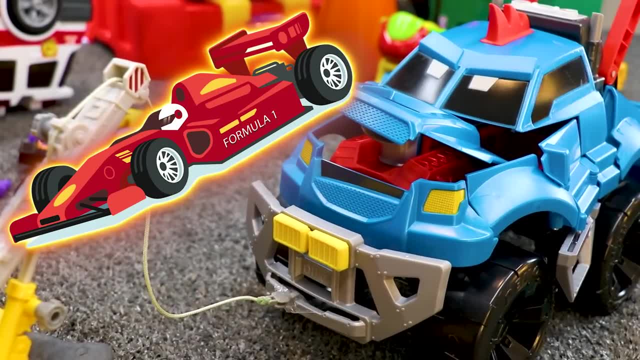 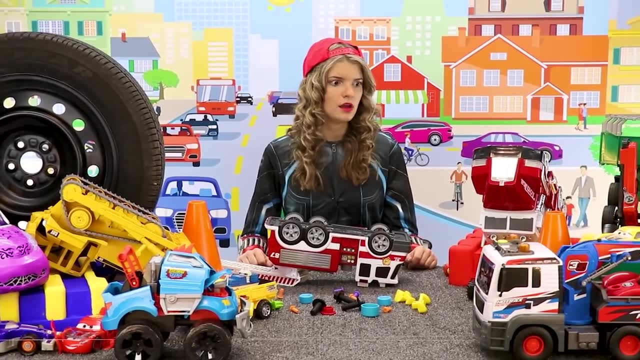 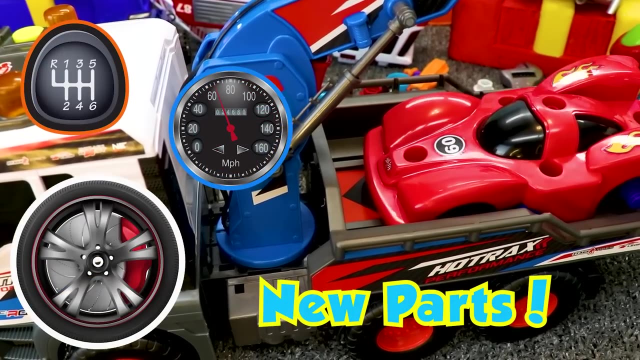 What? And I crashed into a race car. Oh no, That sounds terrible. One more coming. All right, bring her in Race car. you are in really bad shape. I'm okay. I just need new parts. Well, I'm glad to hear that you guys are not in pain. 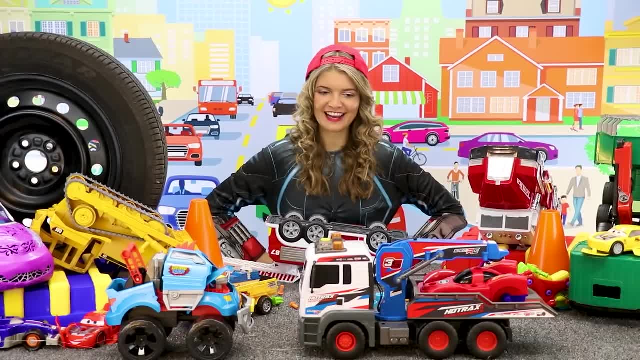 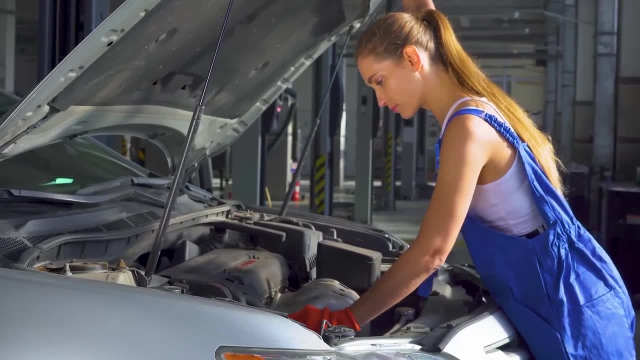 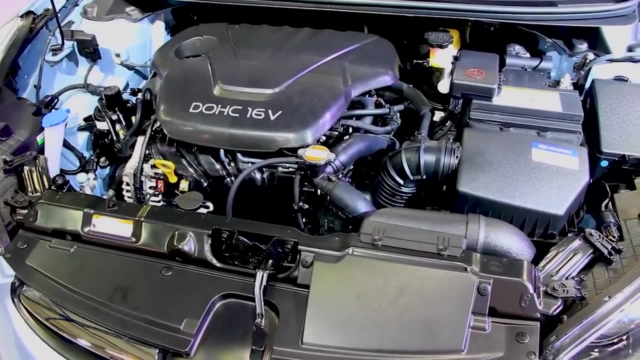 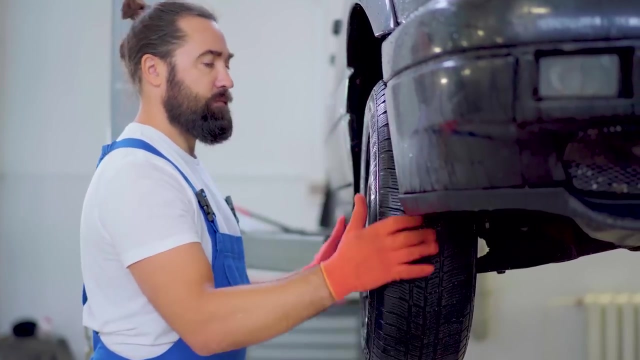 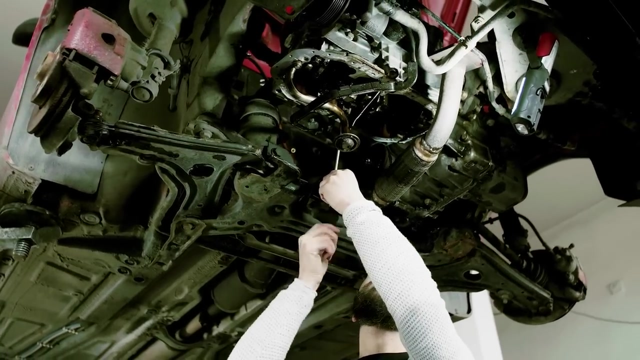 And you've come to the right place to get fixed up: Didi's Mechanic Shop. A car mechanic is someone who's trained to fix vehicles. I've just got to get my car fixed up. What, Yeah, I've just been so busy I don't even have time to fix it. 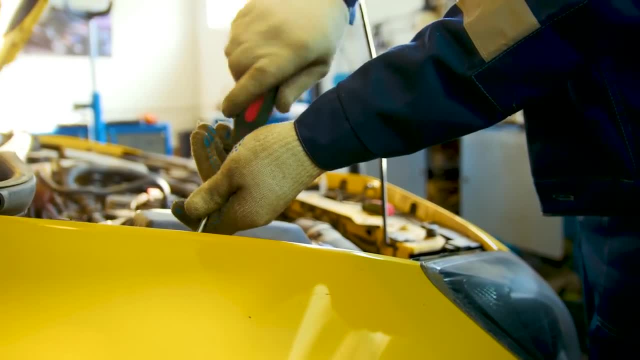 I'll be waiting for you. I'm sorry You're not from here. you got a new car right. I'm a new guy, I'm a new driver and I'm not going to be at the race car for you. 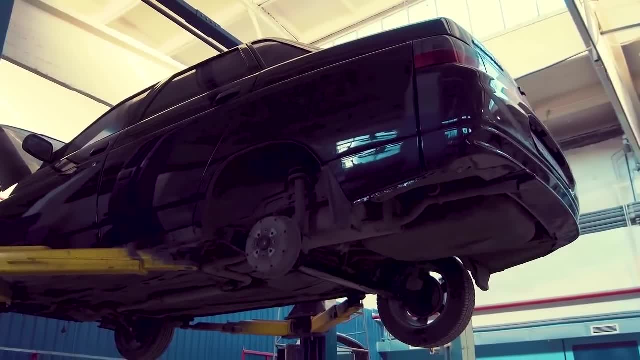 And I'm going to get you a new car. I'm sorry, I don't know if you guys know this, but I just don't know what you guys are doing. You guys are really in a lot of trouble and you're not even driving. 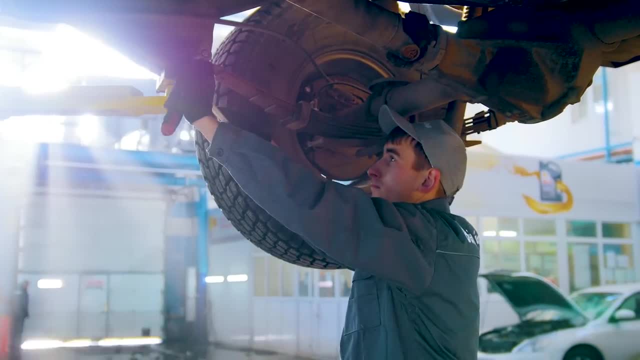 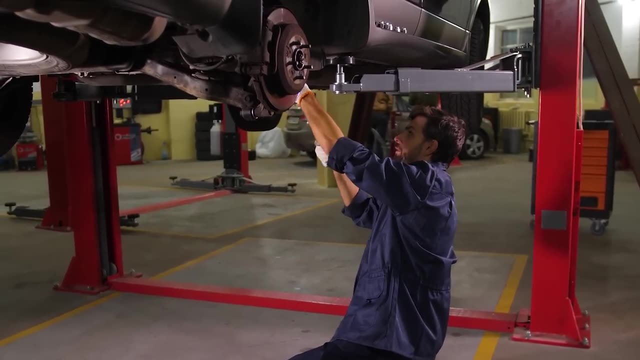 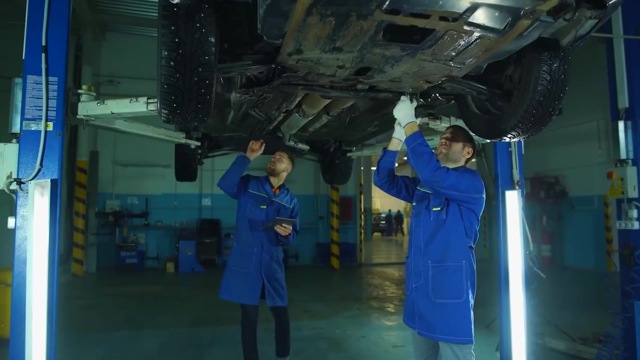 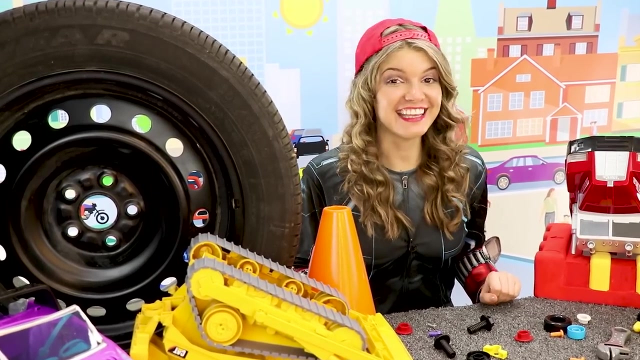 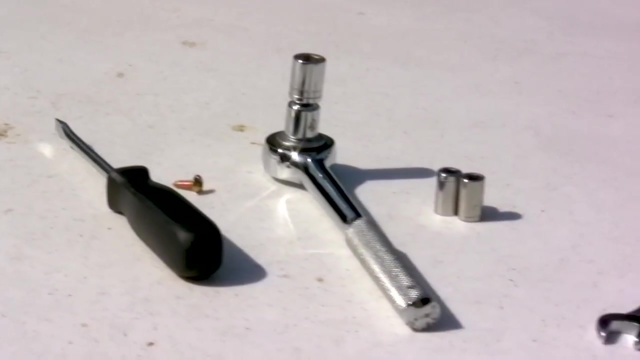 I'm sorry, I don't know what you're doing. I'm just trying to get you in here. Oh, I'm sorry. I'm sorry, I'm not doing anything. First thing we need to do is get our tools. These are all tools. they will help us fix. 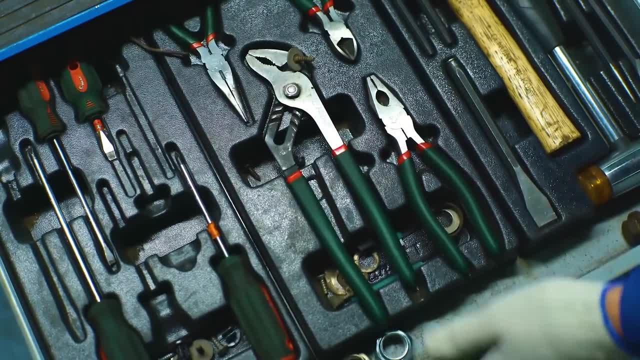 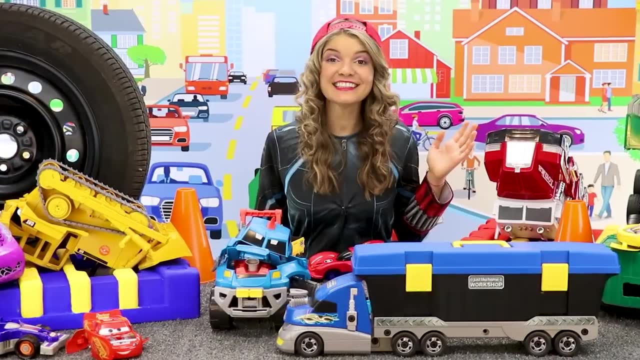 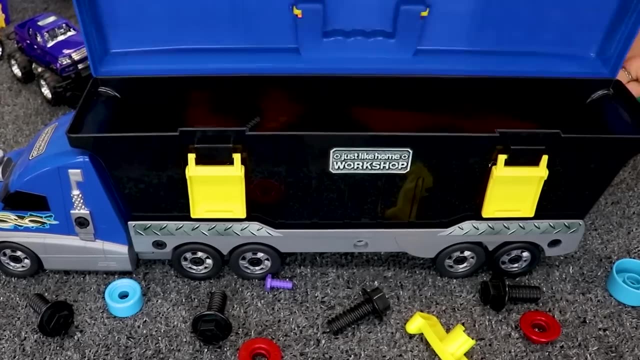 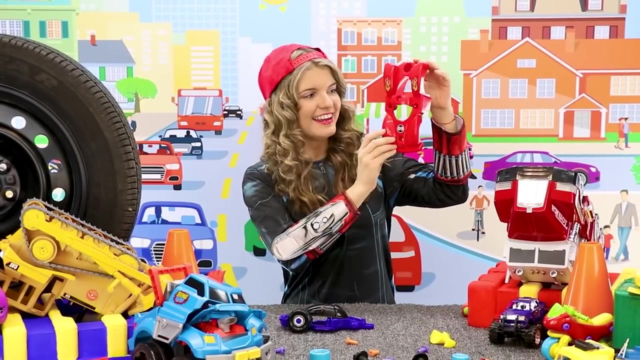 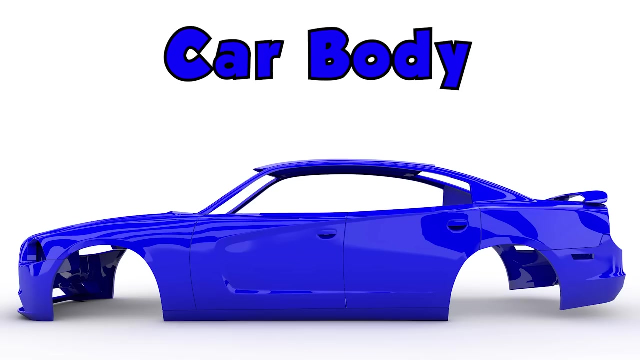 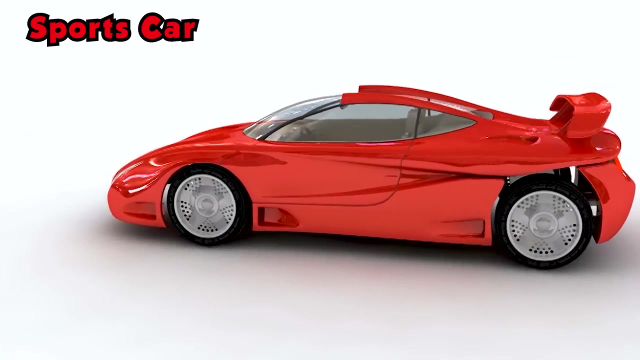 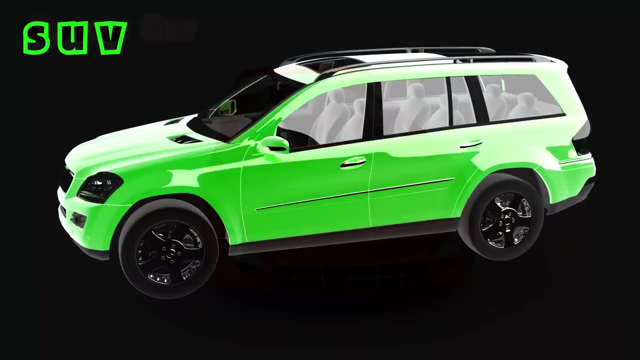 the cars I'm bringing the tools: Didi, Awesome. Our race car has different parts. This red part right here is the car's body, The body of the car. Identify it, Identifies its shape and its style. But different cars have different bodies. For example, the body of this sports car is different from the body of an SUV. 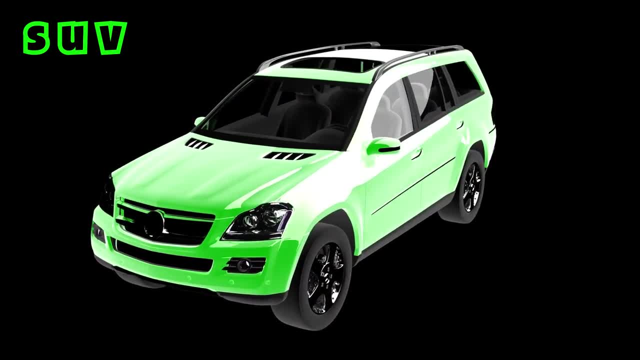 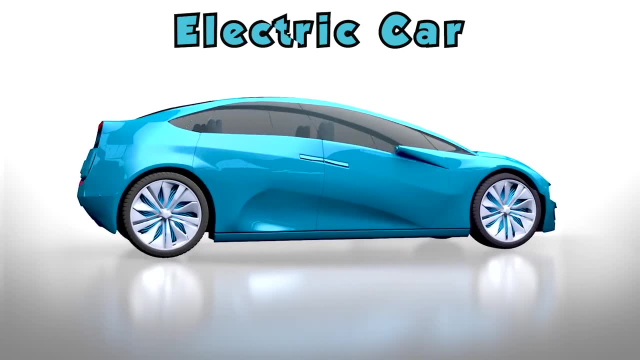 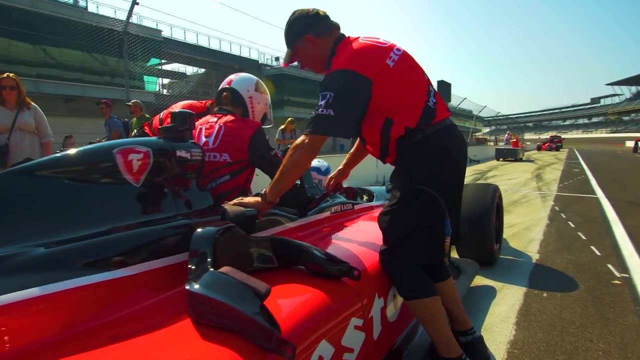 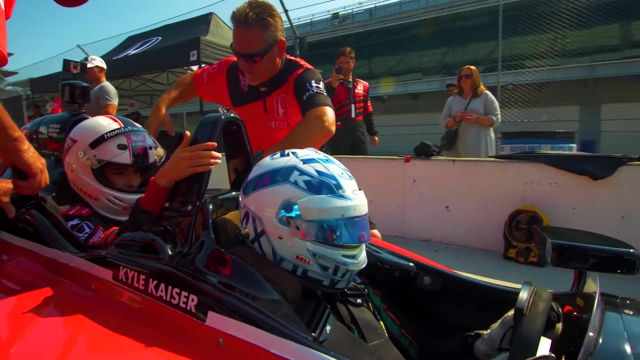 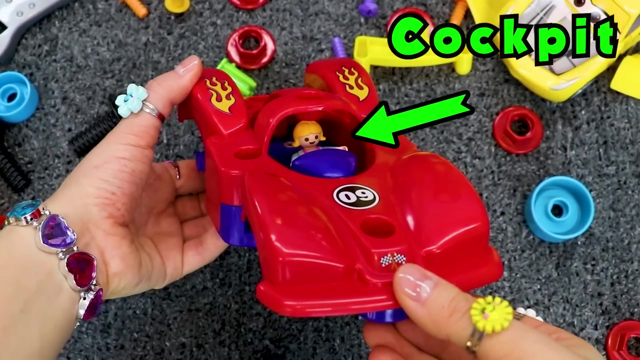 And the SUV has a different body than this electric car. The race car also has a cockpit, Which is the area where the driver sits. In our toy race car, the cockpit looks like this: Our race car has a closed cockpit. That's because it has two windows. 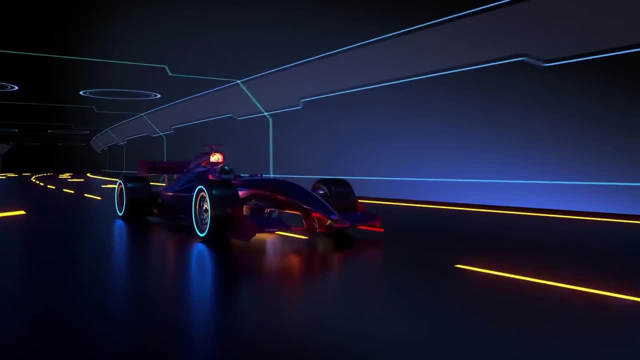 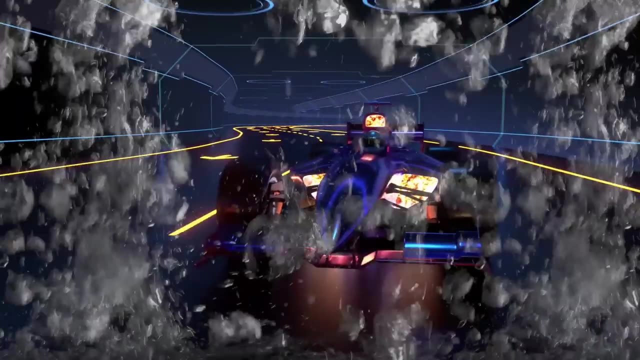 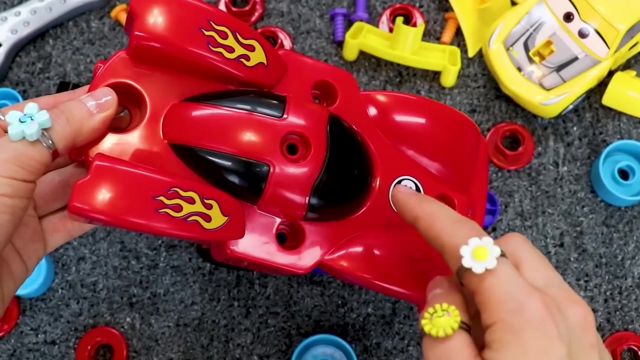 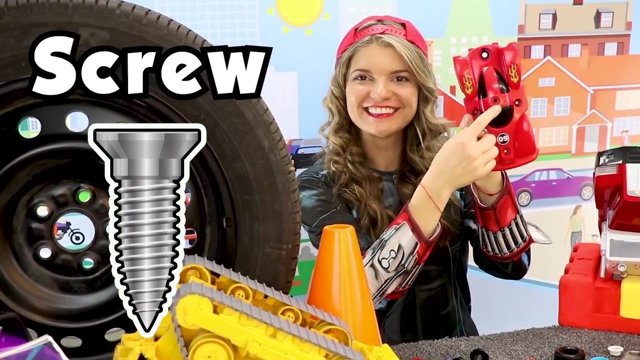 That's why it's called a cockpit. It has this black screen that protects the driver from dirt, debris and rain. Let's attach this black screen to the red frame so it doesn't fall out. To do that, we need to place a screw right here. 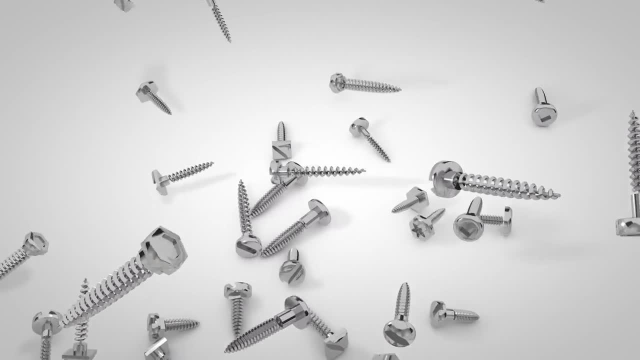 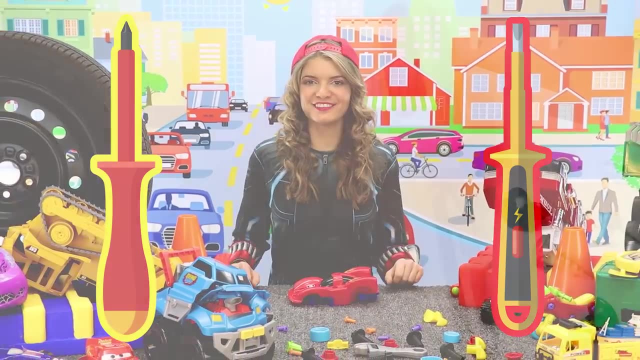 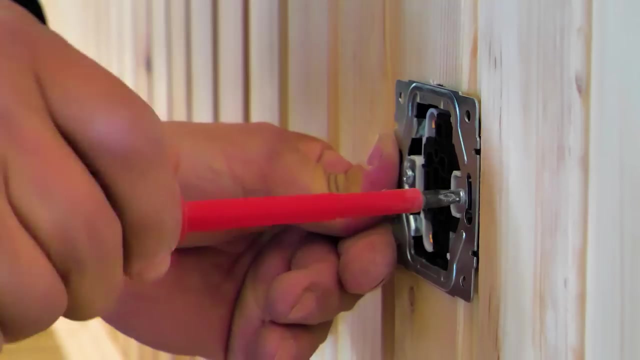 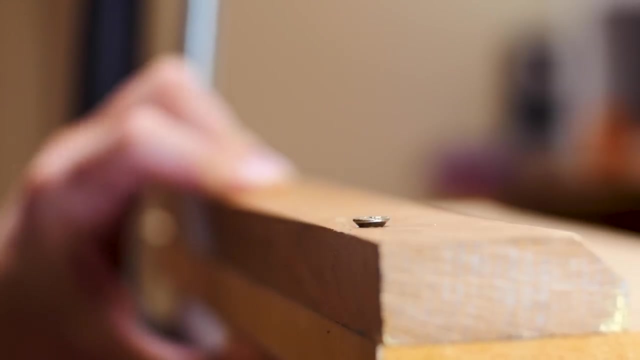 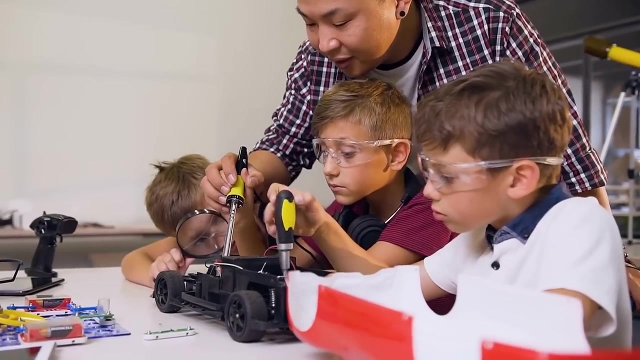 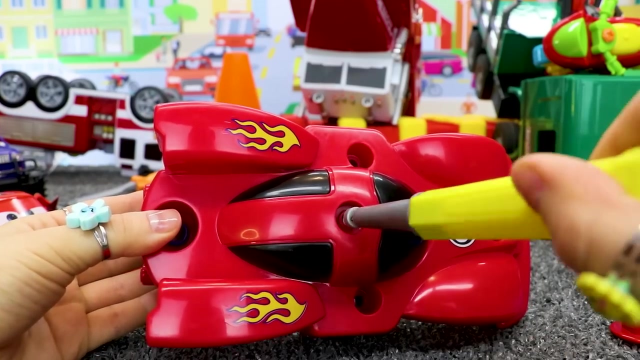 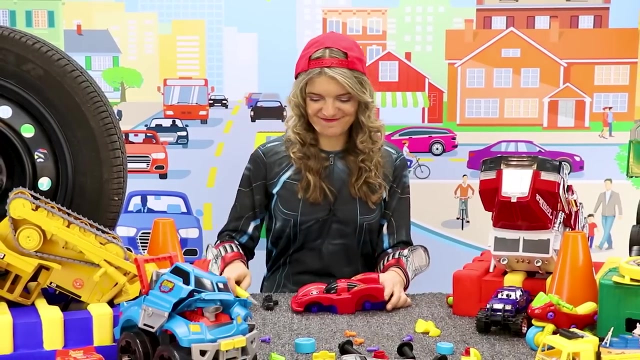 These little things are all screws, And so are these. Now we just need a screwdriver, which is this yellow tool. A screwdriver works like this: Let's attach the black screen to the frame- Awesome. Next, let's attach the front bumper. 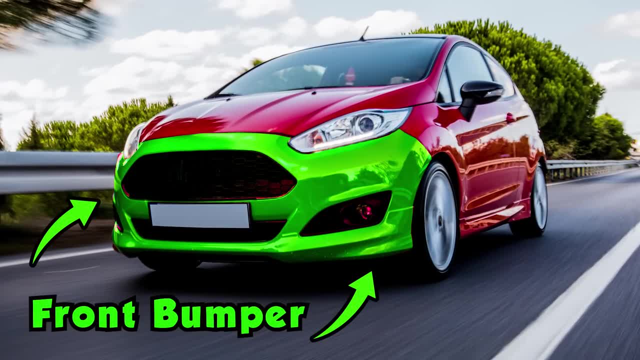 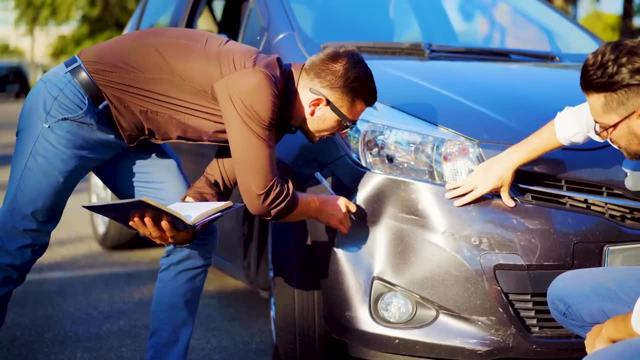 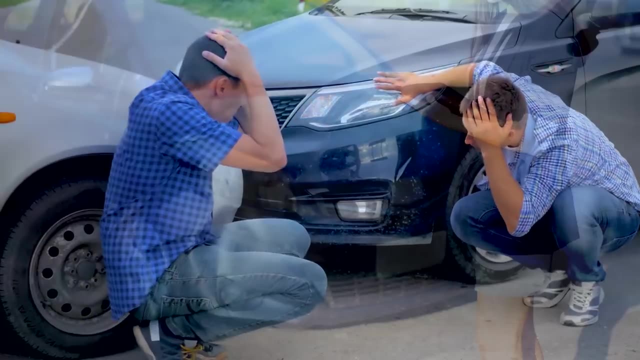 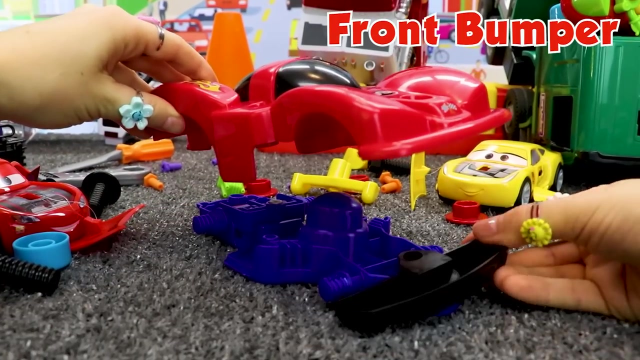 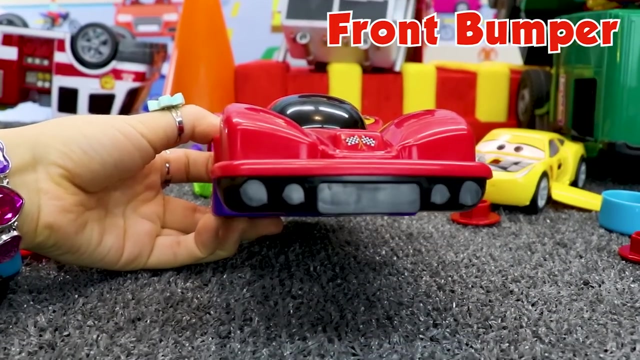 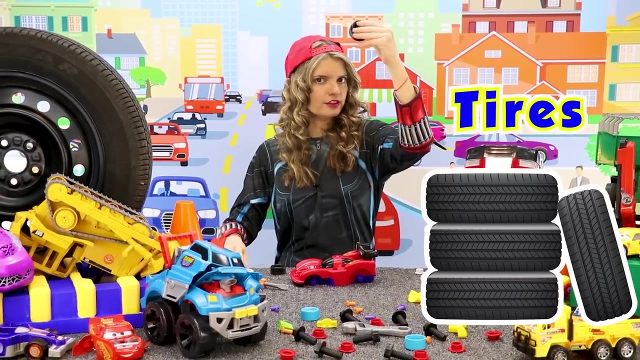 The front bumper is this part of the car. It's usually the first one to get damaged in minor collisions. Let's put in the front bumper. There we go. Alright, guys, almost done. All we have left to do is attach the tires and the rims. 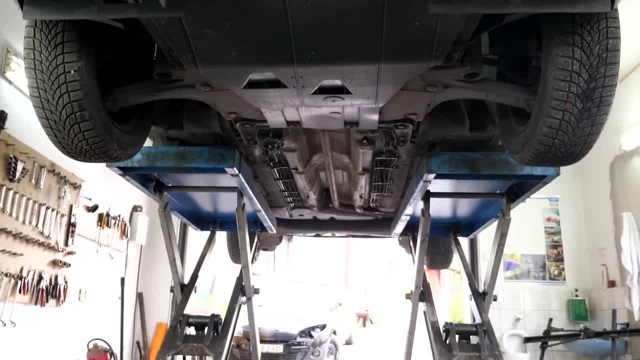 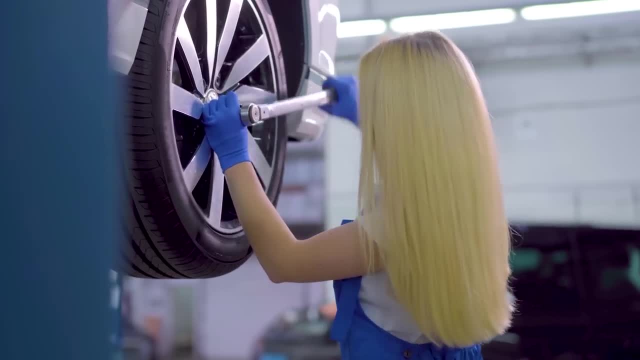 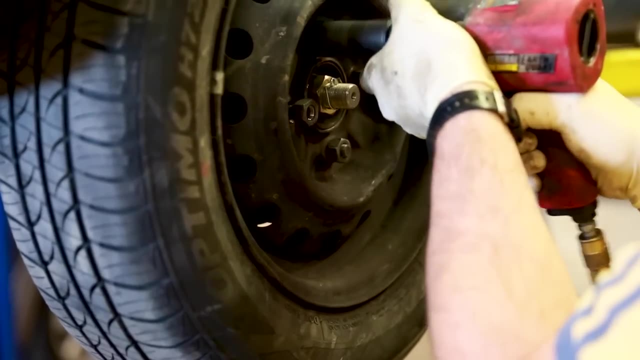 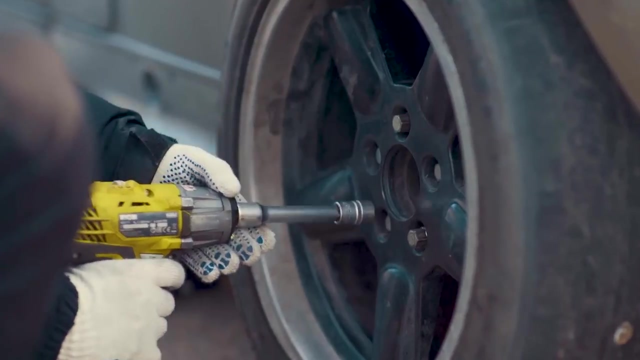 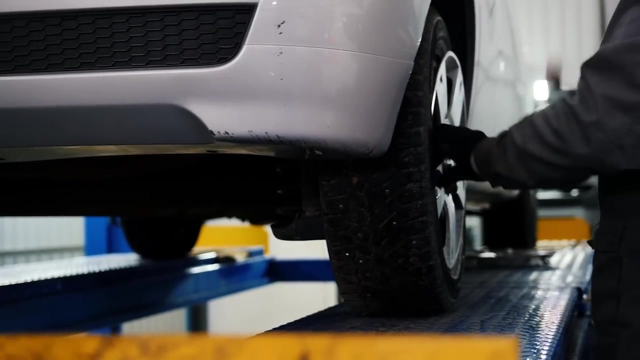 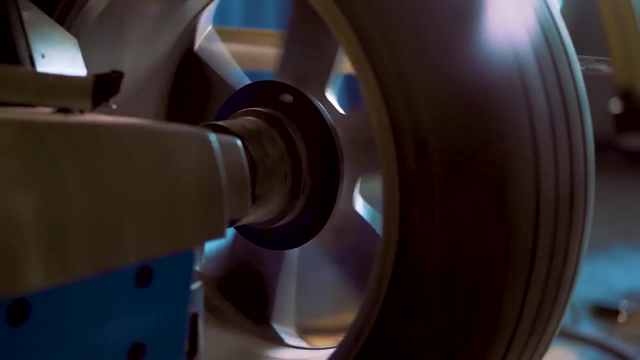 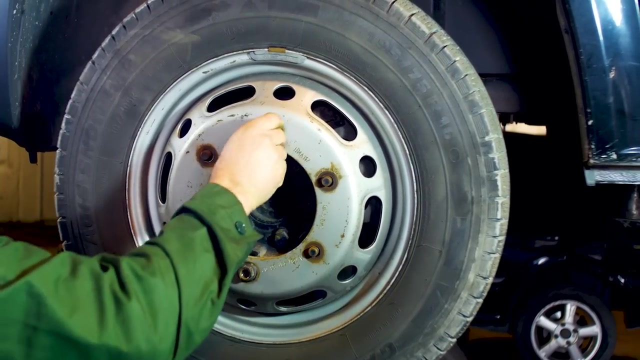 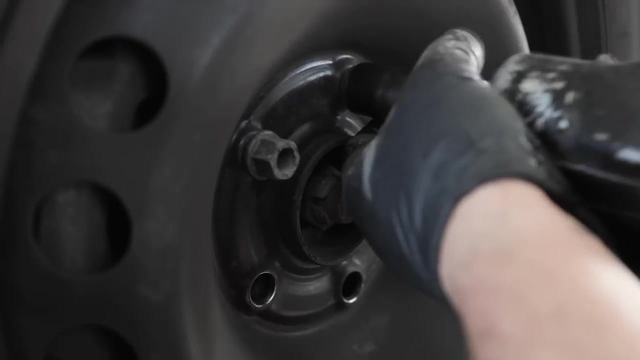 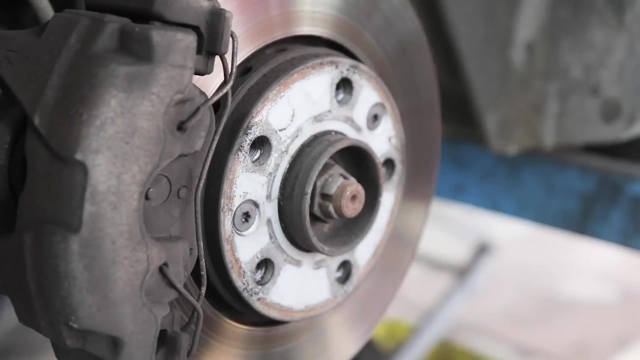 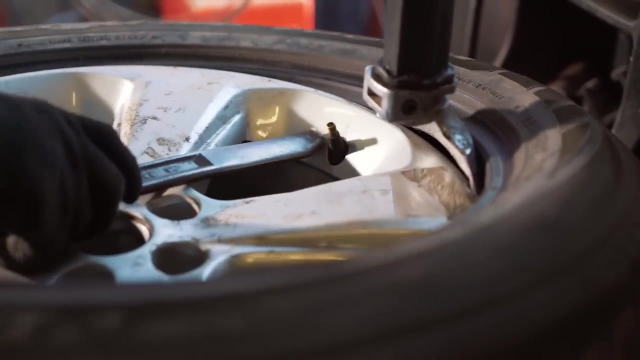 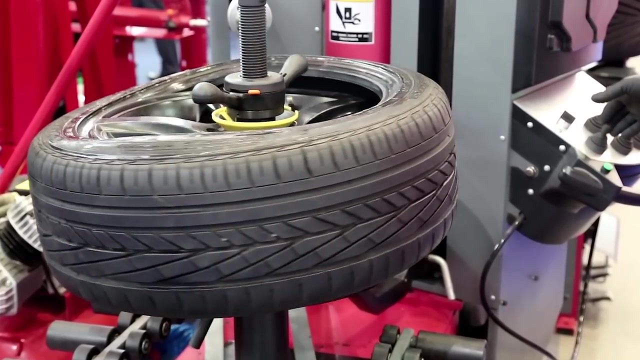 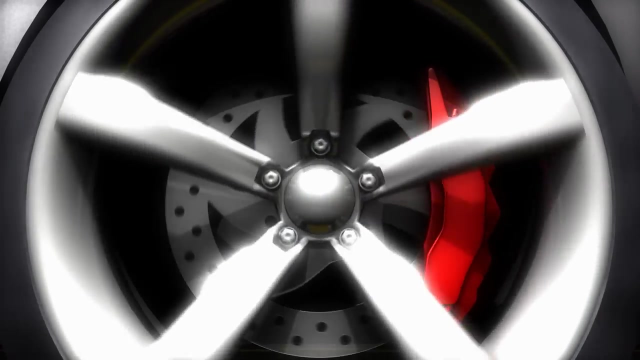 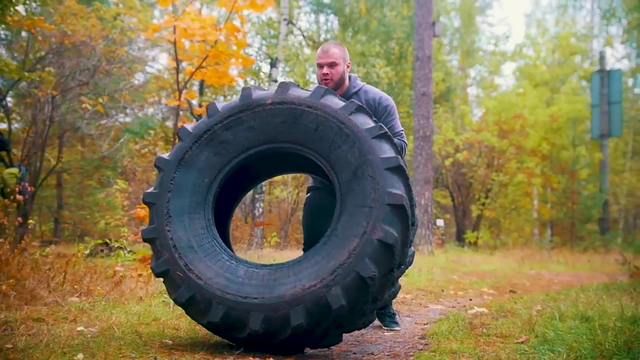 And that's it. Thanks for watching. See you next time. Bye, Bye, Bye, Bye, Bye, Bye, Bye. This is a rim Without a tire. it looks like this, And you already know that this is a tire. 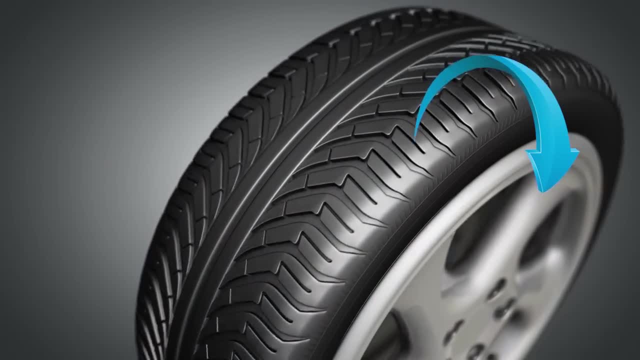 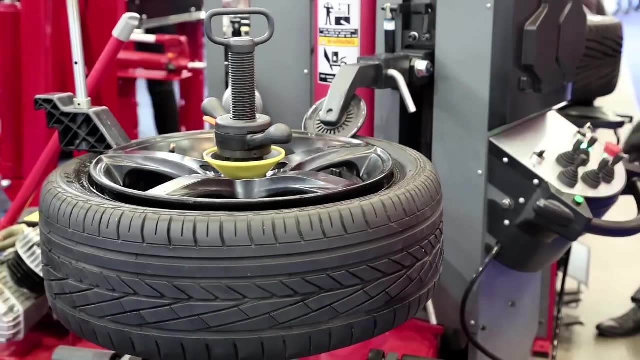 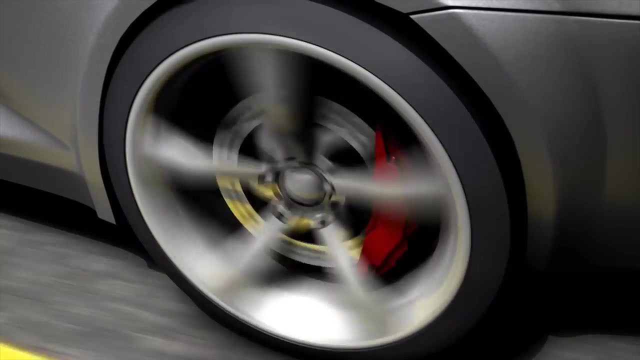 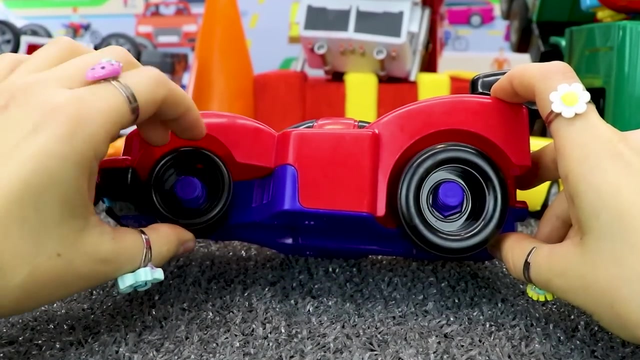 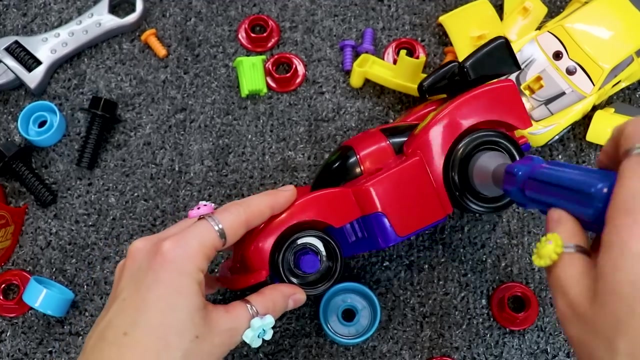 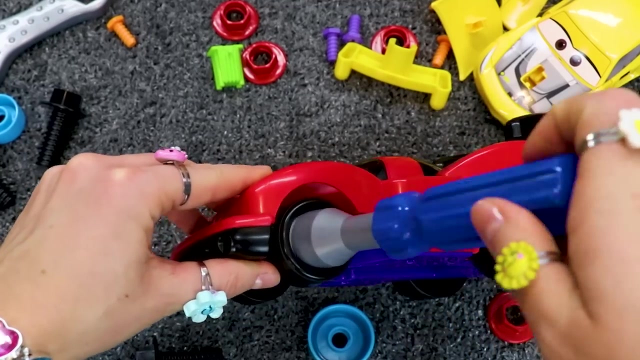 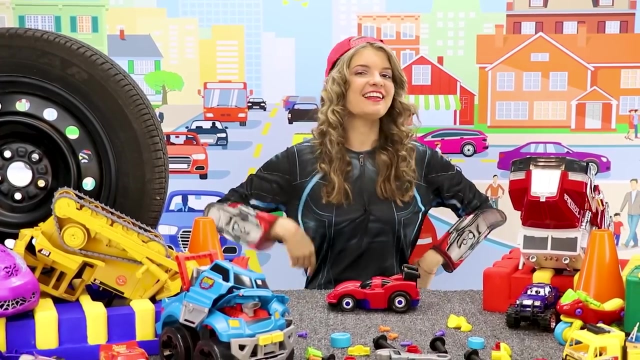 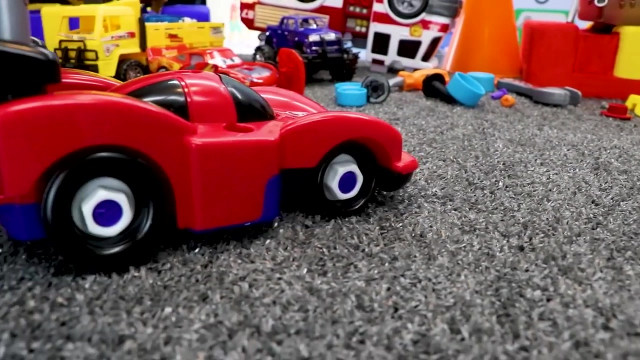 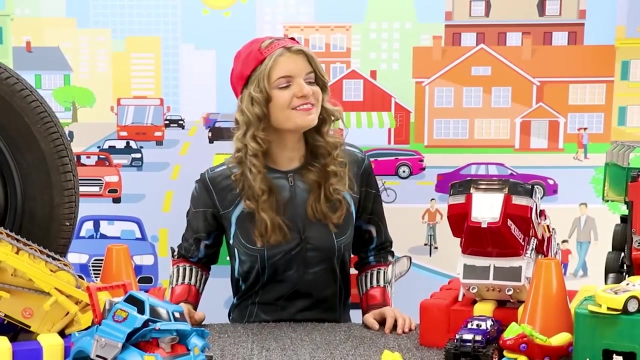 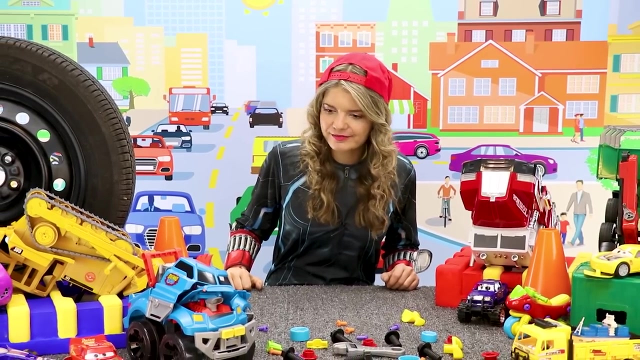 A tire is placed on the rim Like this To allow the vehicle to move. Let's put them on. Well, race car. you are all fixed up and ready to go. No problem, race car bye. Well, can we do? It's finally your turn. We just need to pick you up a little bit and you'll be on your way.